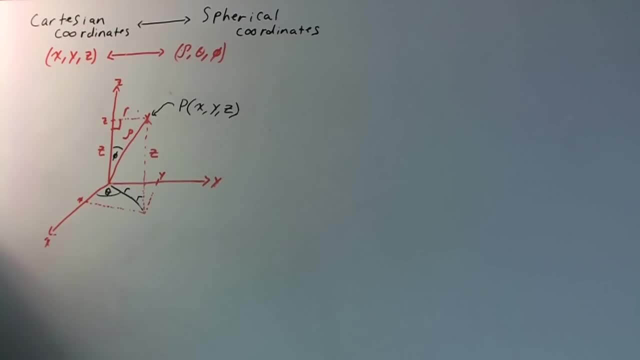 Now, in summary, spherical coordinates are related to polar coordinates by the fact that you just take polar coordinates and add a third dimension And that produces this second angle phi right here. So because they're so closely related, let's talk about what we discovered in the previous video. 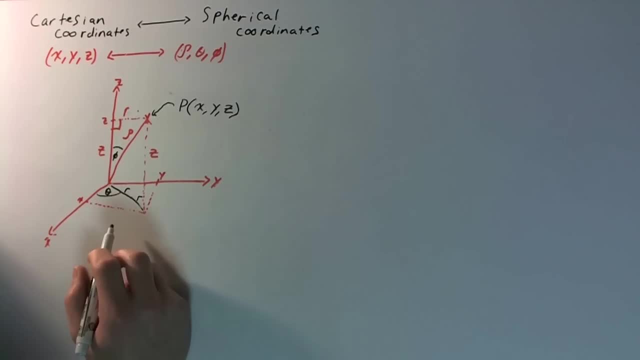 So we know that, If you notice right, this is the same r and theta from polar coordinates and we're just adding a third dimension. So we know that r times the sine theta is going to be equal to y. We know r times the cosine theta is going to be equal to x. 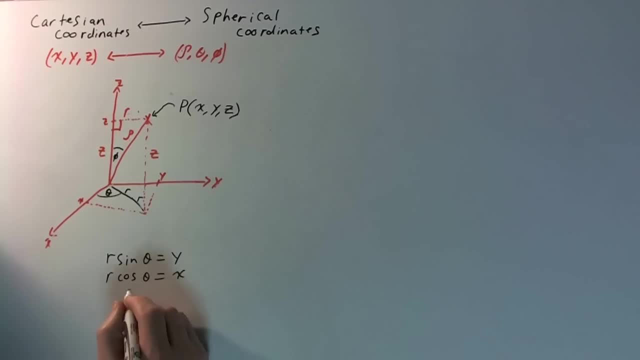 And also, in this case, z. I know this is going to be a real big breakthrough. It's going to be equal to z. Now what does that mean? That means that, basically, you can actually shift the plane up and still have the polar coordinates defined. 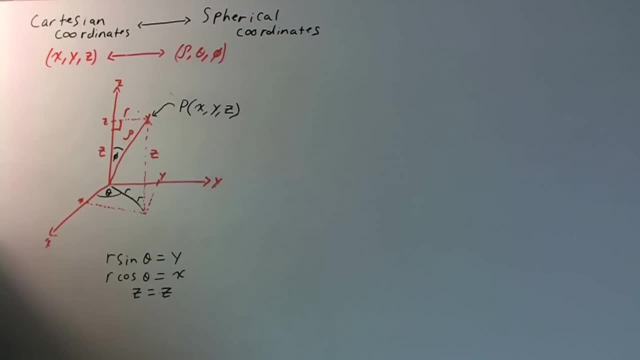 So that's great. You know, we have r defined right, We know theta, But the problem is we need to know rho and we need phi. So let's take this triangle here And expand it and see what we can find here. 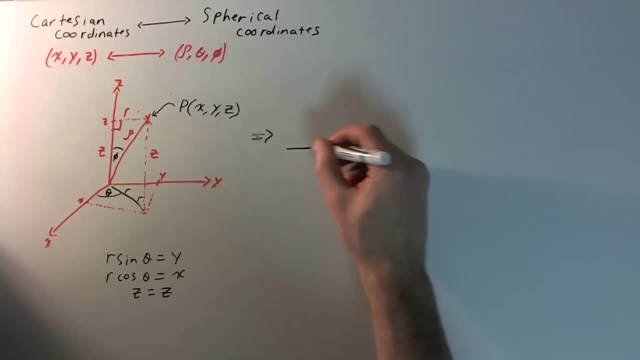 So I'm just going to flip this around here to make it look like If I can learn how to draw a straight line, that would be great. There we go: Right triangle. Now, in this case, this is the angle. phi right. 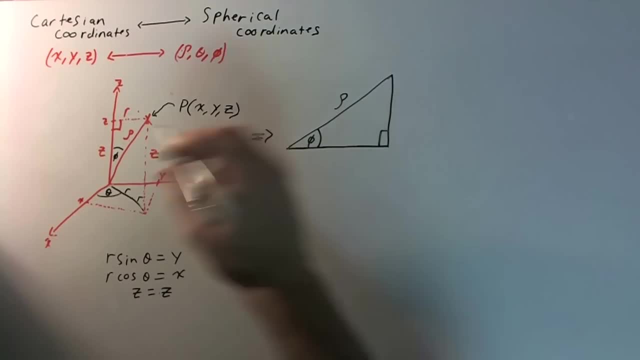 This is rho And the height. The height for this triangle is r, right The same r in polar coordinates And this Right The x on the bottom here, or what would normally be x, is z. So using trigonometry and our trigonometric functions, we can actually solve this angle as a function of the hypotenuse and the two legs. 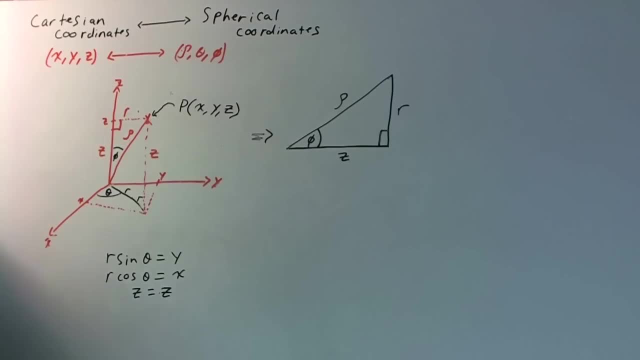 So let us do that. So let's, Let's see. We know that the sine of phi right is going to be equal to well, if you remember SOHCAHTOA, right opposite over the hypotenuse, right r over rho. 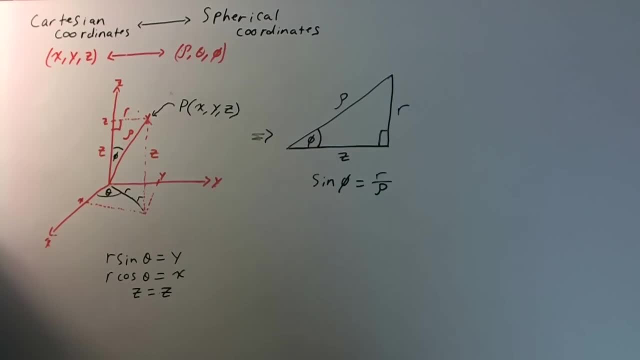 And we also know the fact that rho squared is going to be equal to r squared plus z squared right, And we can obviously solve this. So if you solve for this, get rho. it's going to be equal to the square root of r squared plus z squared right. 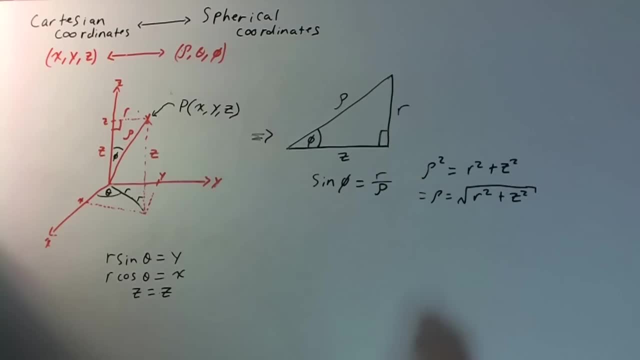 But the thing is we know what r squared is right because we know from polar coordinates that r squared is just x squared plus y squared right. So that's just this: r is going to be equal to the square root of x squared plus y squared right. 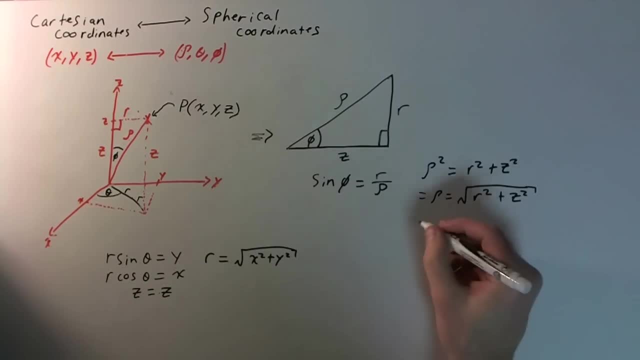 This length here. So we just plug this in and we can find that Uh, row is going to be equal to x squared, y squared plus z squared, right? So that's great. Now we know the length of row in terms of x, y and z. 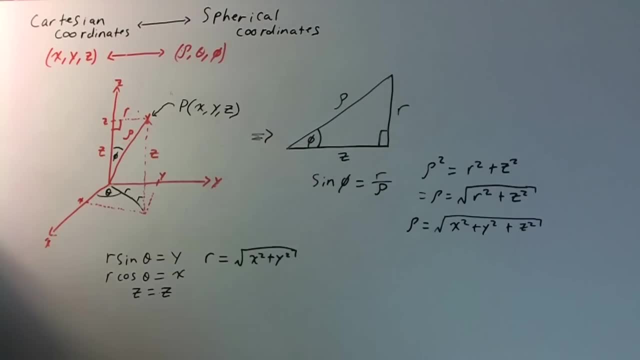 Perfect. Now we need to know phi in terms of x, y and z, right? So if we solve for r, we get the fact that let's do this in a different color here. Let's get rid of this. 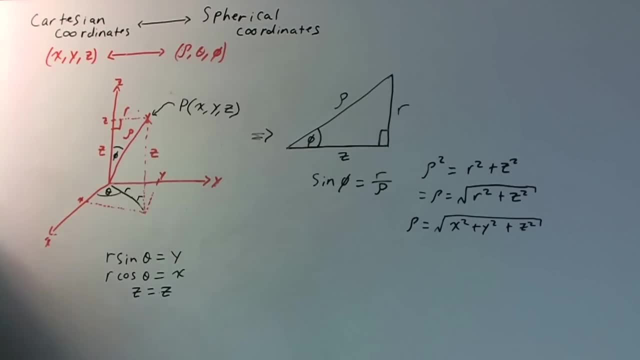 Give myself some room here. We know that if we solve for row, obviously multiply row by both sides. we know that r is going to be equal to row sine theta right. Excuse me, sine phi, There we go. R sine phi. 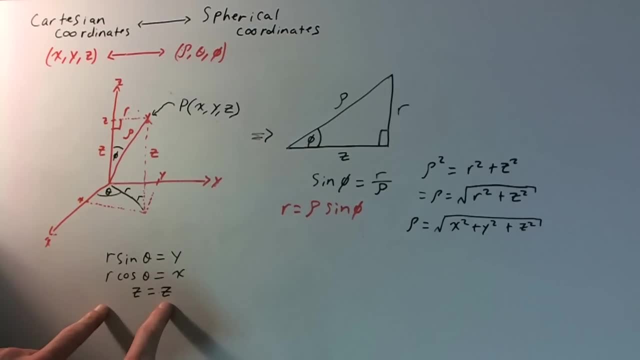 And so since we already know in polar coordinates what r is right r is here, we can actually plug this r, which is the same r, into this equation and have everything defined for x and y. So let's do that, and we'll deal with z in a second right.